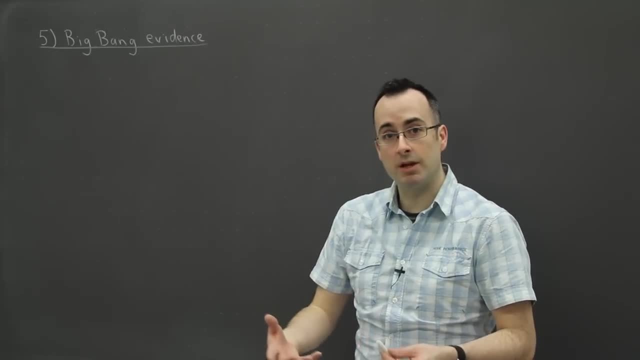 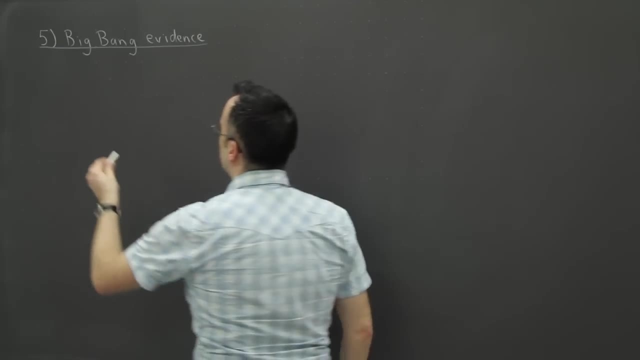 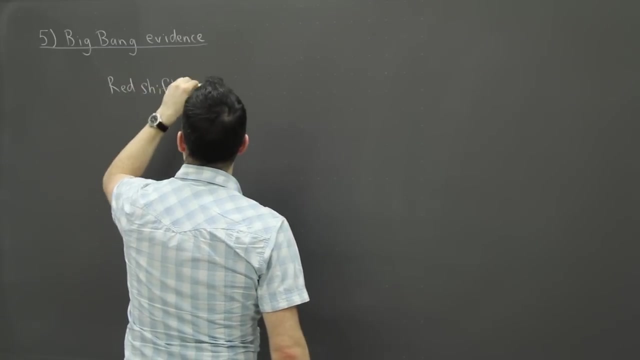 evidence certainly seems to point to that. So if someone else has a theory of the universe, it had better explain these two very important pieces of evidence. So one of them is redshift- I'll say redshifted- galaxies. Maybe this will be a little bit nicer to look at here. So what do I mean by redshifted galaxies? 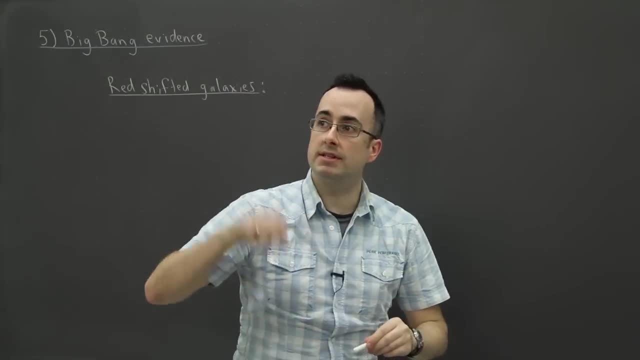 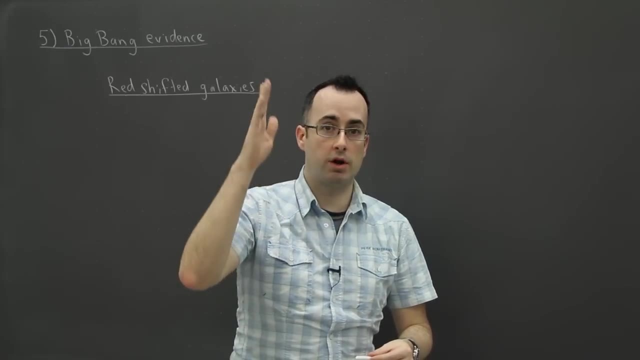 I mean that if you look out into the sky, you not only see lots of dots, which are stars, but if you use a high-powered telescope or even on a nice sky, if you know where to look, you can actually see, for example, the Andromeda Galaxy in the Northern Hemisphere, In the Southern 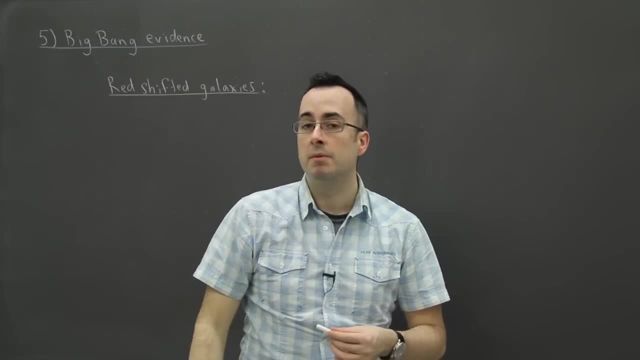 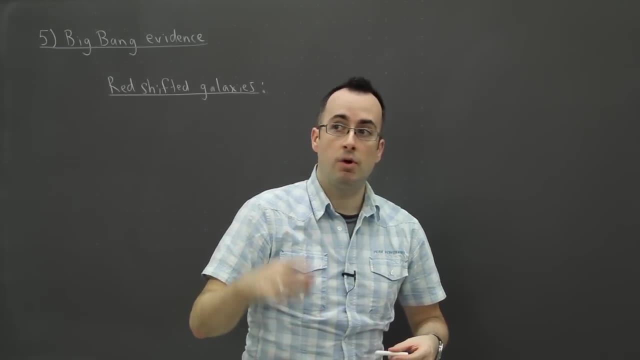 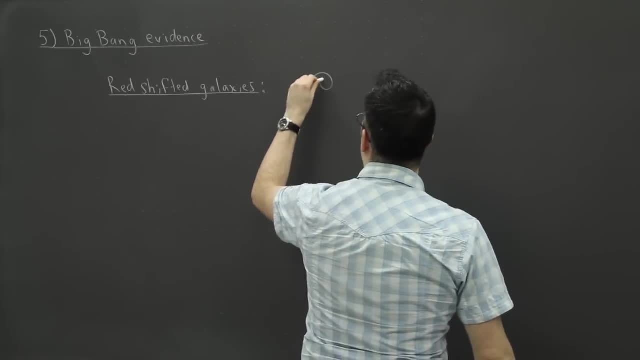 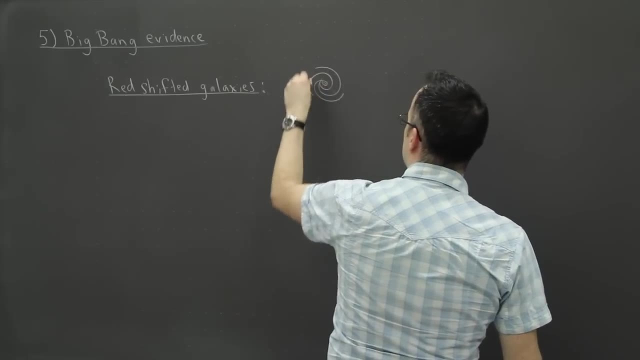 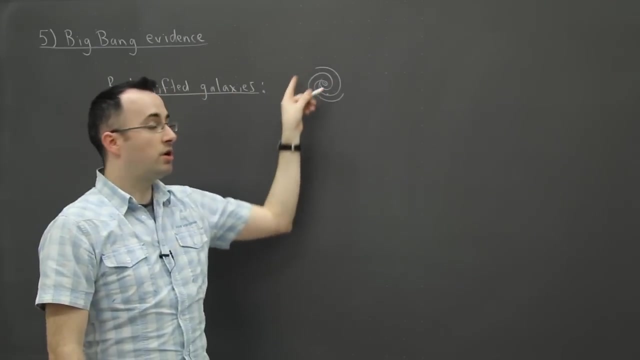 nice galaxies. so you know galaxies might look like. you know a nice spiral, for example, some sort of really cool-looking. you know galaxy like this. You know it's got billions and billions of stars in it. Well, we're in one. We're about two-thirds of the way out, And our galaxy we call 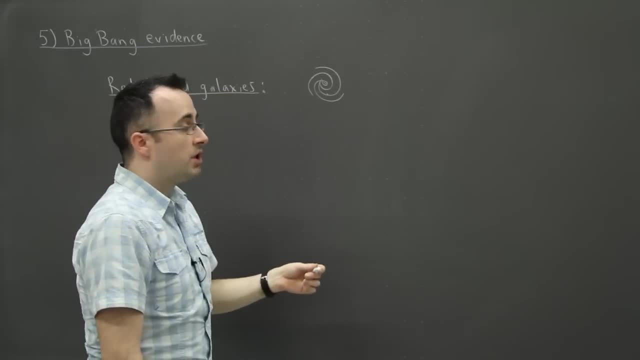 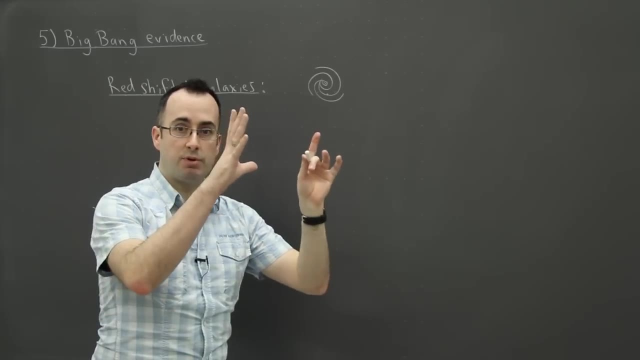 it the Milky Way Galaxy, But there's lots and lots of other galaxies. So it turns out, when we take the light from a galaxy, we're not going to be able to see the light from a galaxy, We're going to be able to see the light from a galaxy. Not only does it make a nice, pretty picture, because that 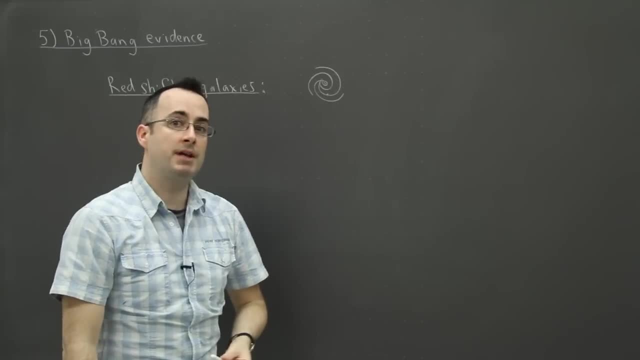 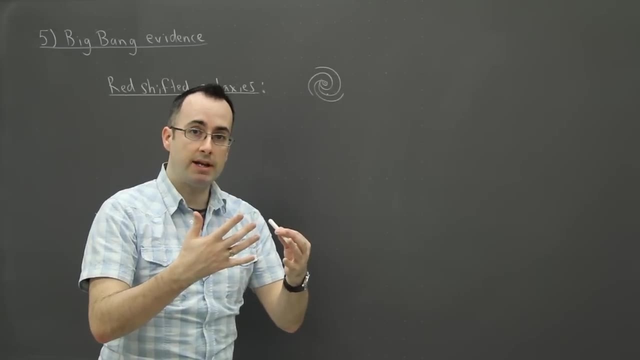 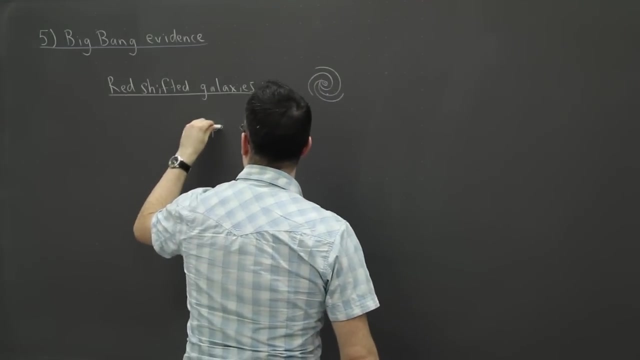 might be something that you use to- you know, sell posters- but what scientists really want to do is to take a look at the spectrum of light. In other words, you take the light and you break it up into its different wavelengths, So you end up with: so look at this, Here's a spectrum of a star, maybe. 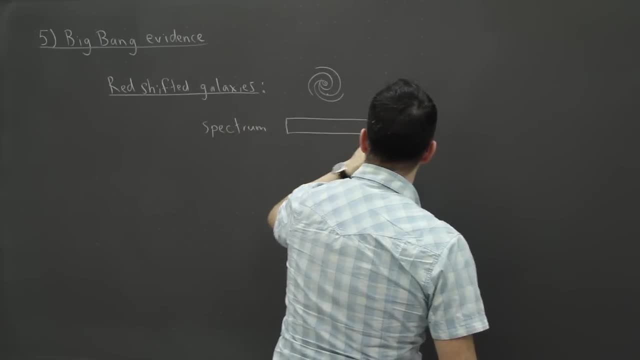 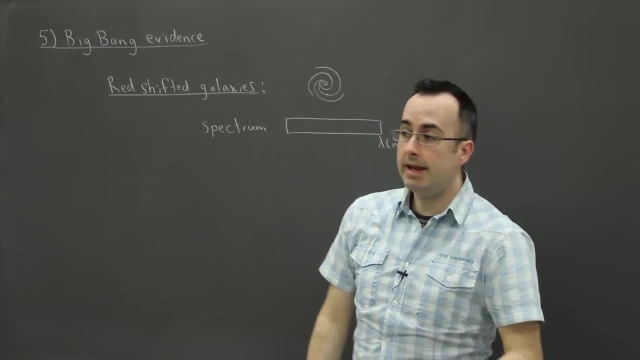 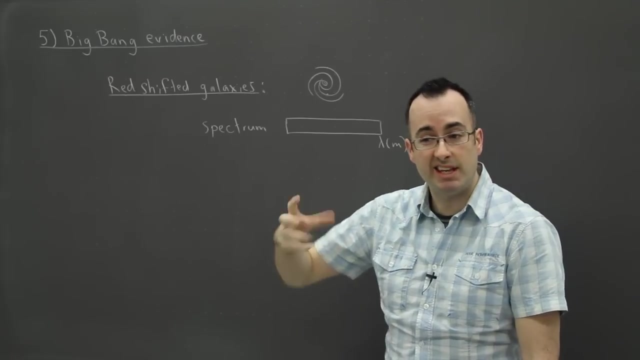 So this is what would end up happening. You'd actually break it up and this would be sort of a graph of wavelength in meters. Now what happens is this: If you take any element and you heat it up, let's say you zap it. So let's say you take I don't know some hydrogen gas and you heat it up. If you do that, 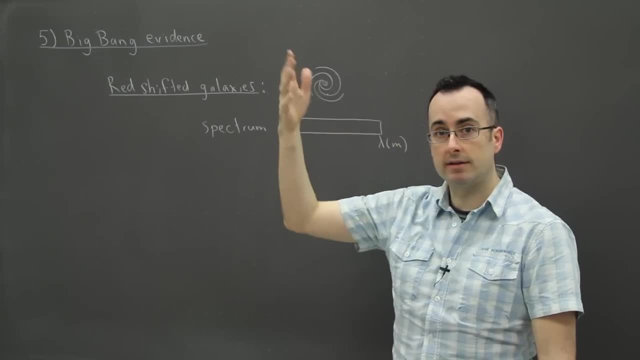 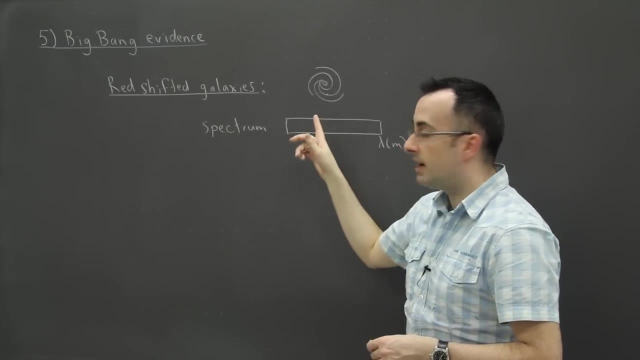 you're actually going to see if you break up that light that you get, because it's going to give off light. If you take the light from helium, for example, or hydrogen or some other gas, and you break it up into its, if you look at its spectrum here. in other words, 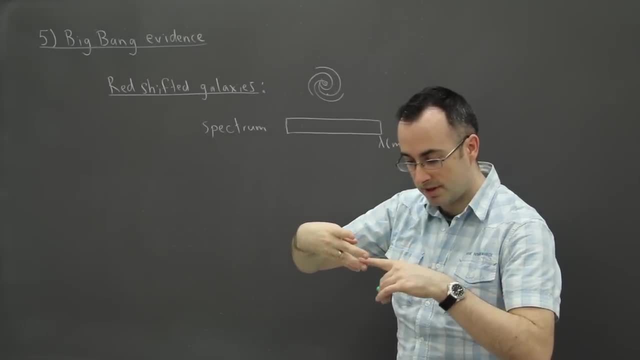 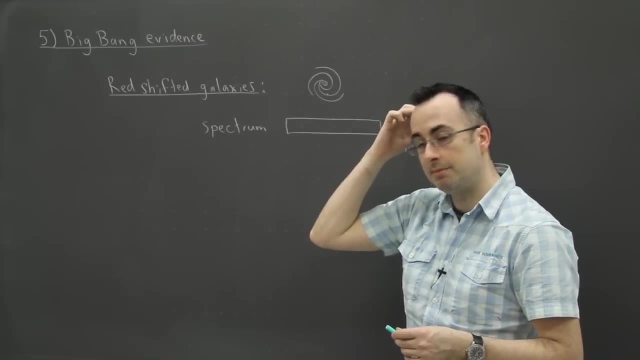 you put it through a prism and you sort of split up the light into all the different things that are actually going on. you're going to see very specific lines Now. they could be absorption or emission lines, but let's just look at these lines. So let's let's just say that some element has a very 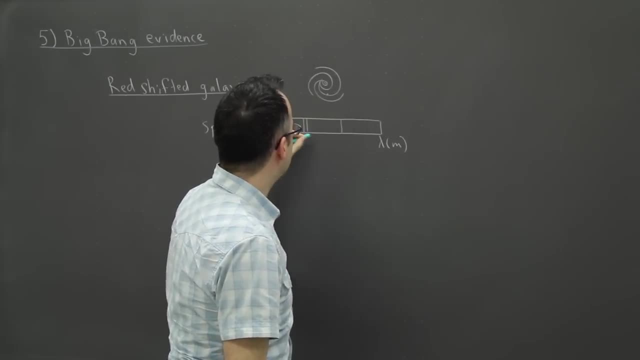 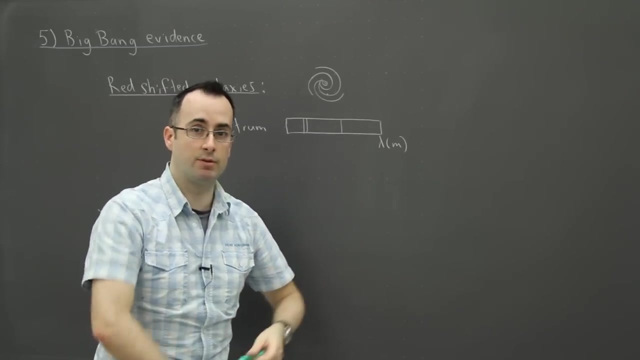 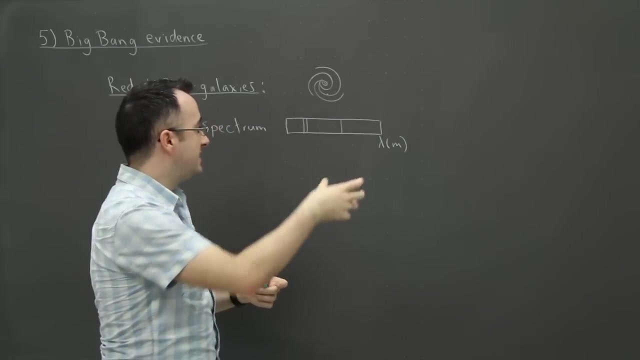 specific fingerprint. Maybe it does this, Maybe it's got like two here and then one here. Well, this you can see in a lab. You can do this when you're still, so to speak. What we do, then, is we take the light from a galaxy, or even from a close-by star, and we see these same patterns Because of that. 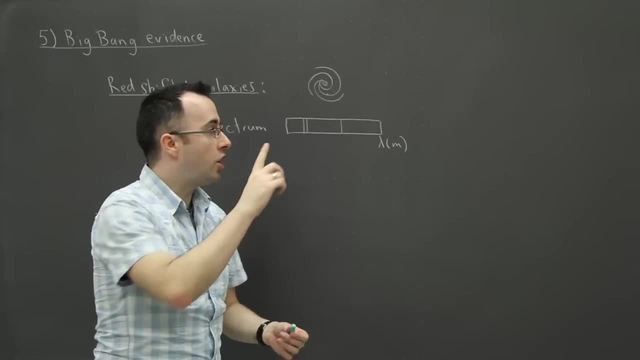 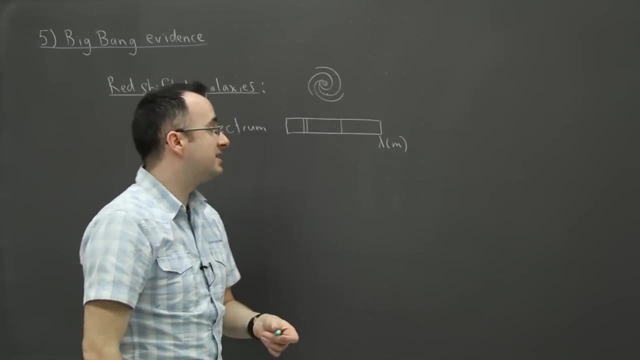 then it's like a fingerprint. Then we can know: aha, this star has blah, blah, blah, and it may be hydrogen and helium and whatever else. Well, the same thing happens with galaxies. We can see the spectrum of light from a galaxy and it may match some elements that we know well here on Earth. 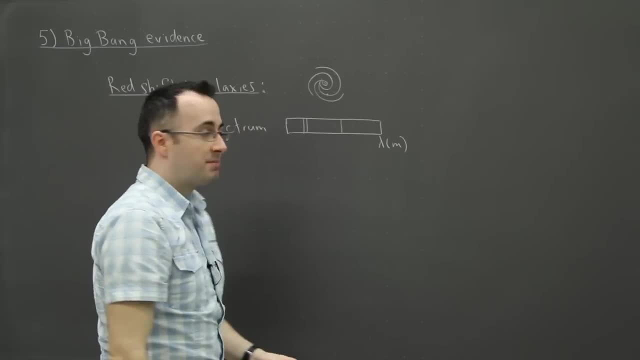 But there's a problem, or maybe not a problem, but something exciting. The spectrum of light from a galaxy is very similar to the spectrum of light from a galaxy. But there's a problem, or maybe not a problem, but something exciting. 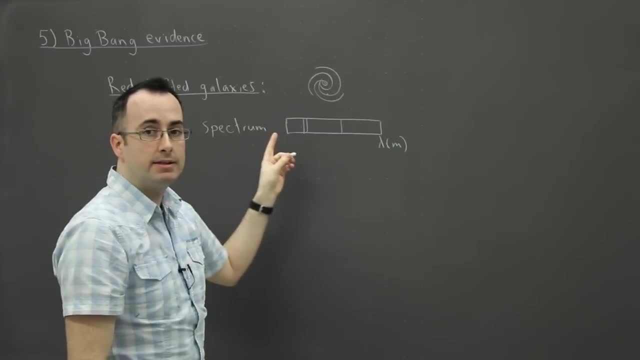 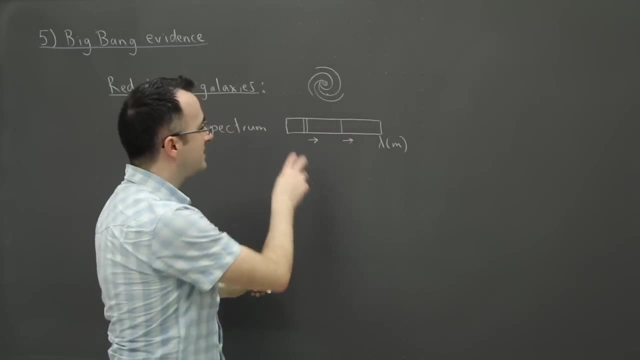 The spectrum of light from a galaxy is very similar to the spectrum of light from a galaxy. So when we look at the spectrum, in other words, these lines that you get from a galaxy- almost all the galaxies we look at- the spectral lines seem you know. so we see the same pattern, but it's like all of them are just shifted a little bit to the right. 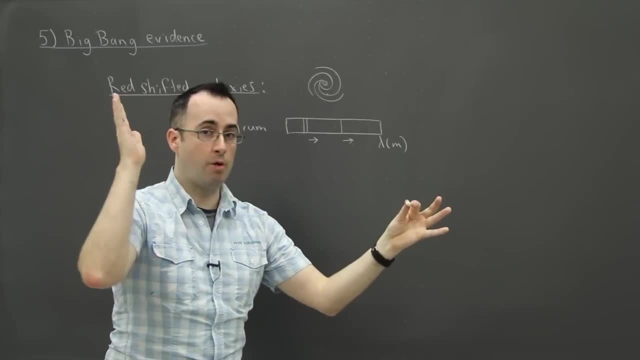 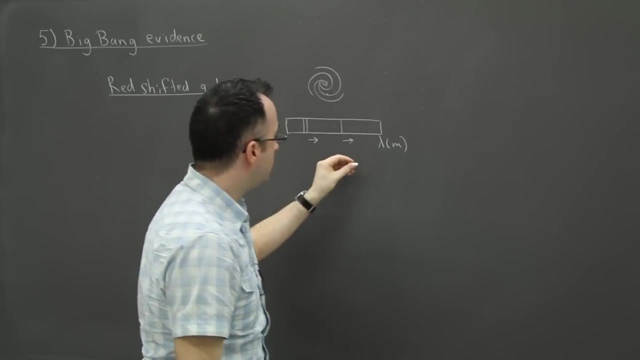 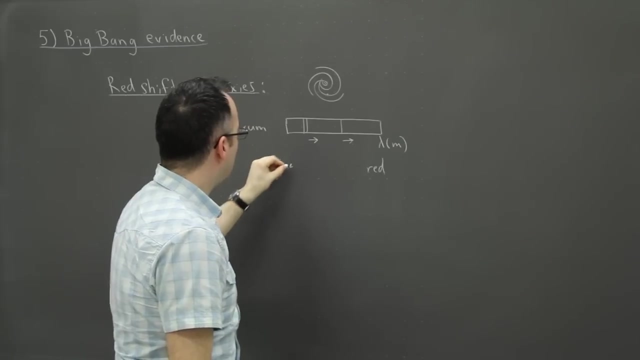 That just seems to be no matter where you look. look at almost any galaxy you can imagine. take a look at it. they do this, And so the explanation is that this is some analogy to the Doppler effect, And what happens is we call it red shifted, because these lines are shifted towards longer wavelengths, so we say they're redder. 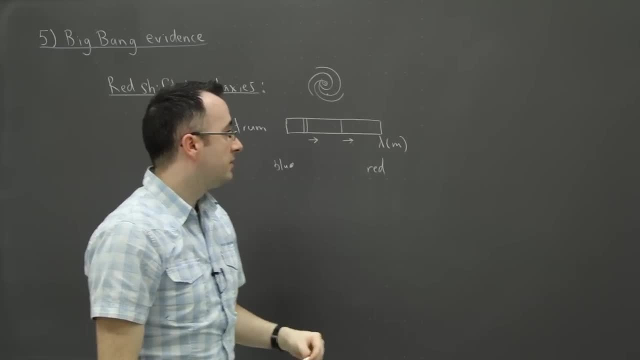 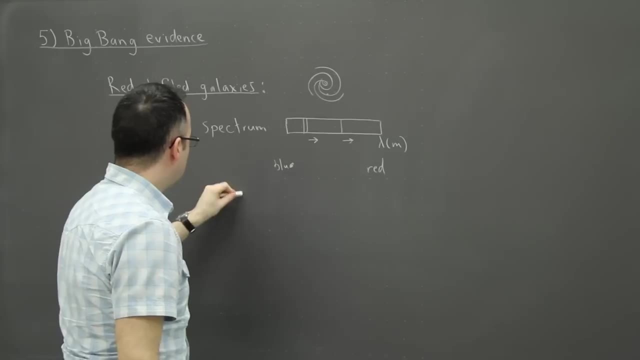 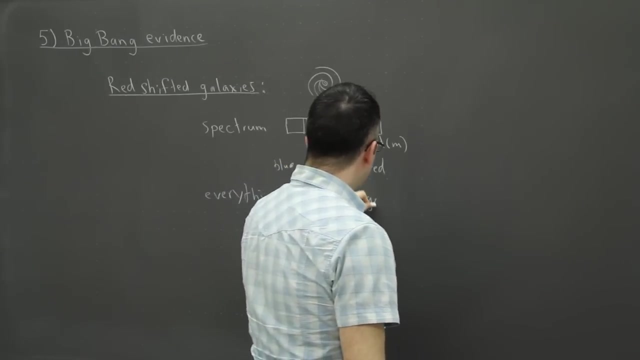 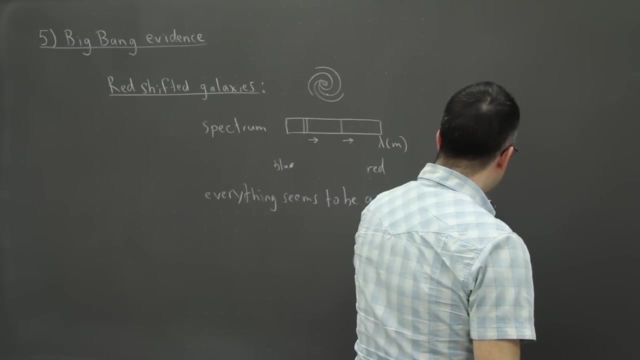 So almost everything we see is red shifted, And what's important is that the conclusion means that everything- oops, I better use a nicer piece of chalk here- everything seems to be going away from us, And that's because if you take light, something that gives off light, and you send it away from you, the 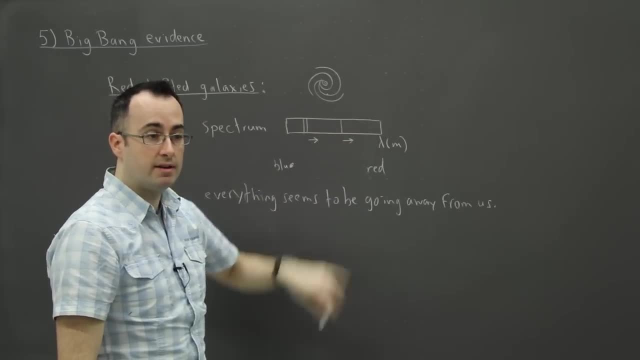 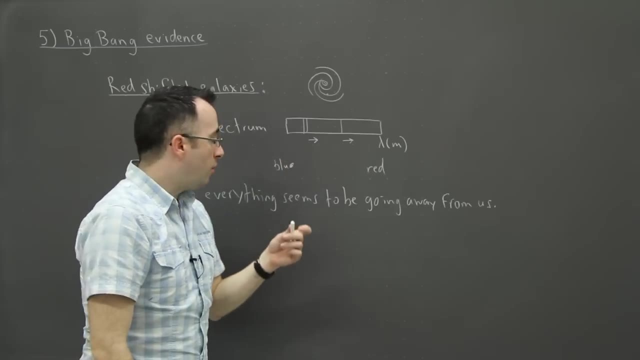 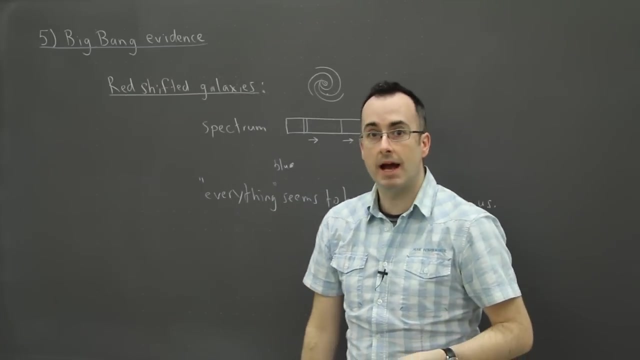 the spectra lines will actually be shifted towards the red. In other words, when we see something red shifted, we can infer that it's going away from us. Now, when I say everything, not quite, There's a few exceptions. In fact, one of the closest, well, the closest galaxy to us, 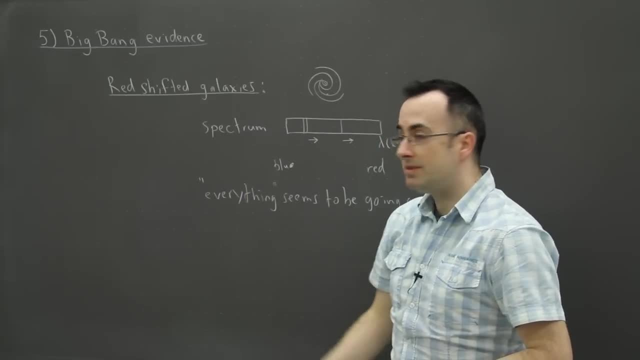 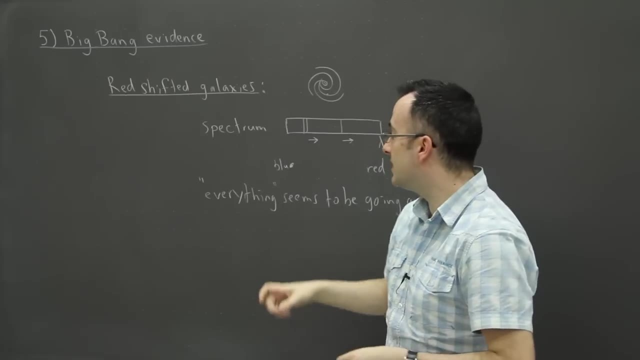 it's a really big one called the Andromeda Galaxy and that one's actually coming towards us or we're coming towards it. it's hard to tell, But basically we're coming towards each other. In other words, Andromeda Galaxy is actually blue shifted, which means it's coming towards us. 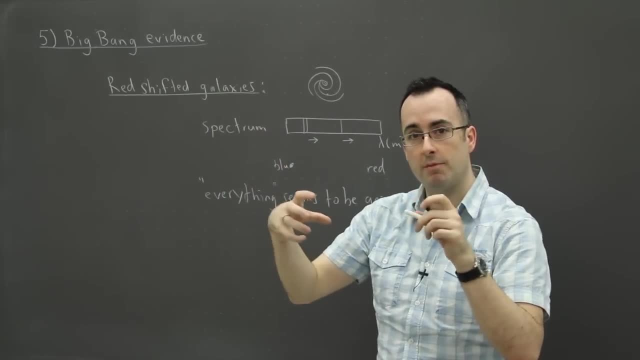 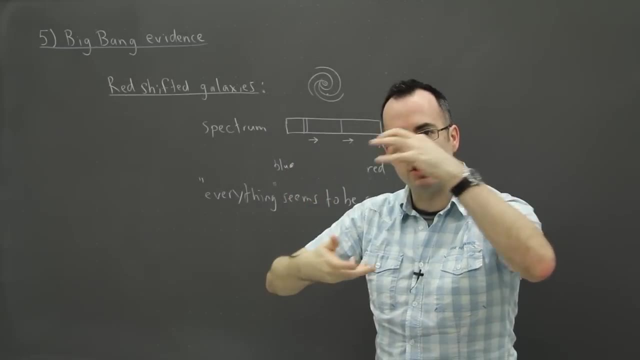 But with very few exceptions. there's only a few galaxies that are coming towards us, and they're all our local, neighborhood ones. The explanation is that we're all so close together, we're all attracting each other, so we're all sort of 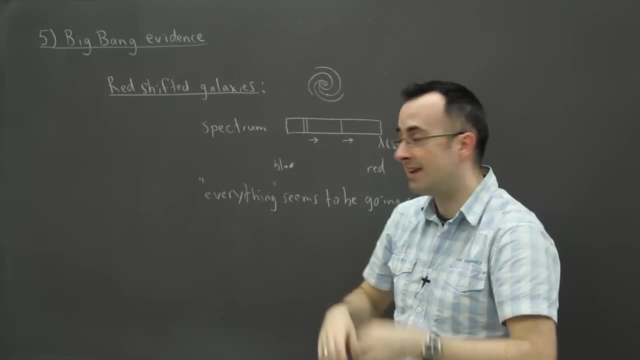 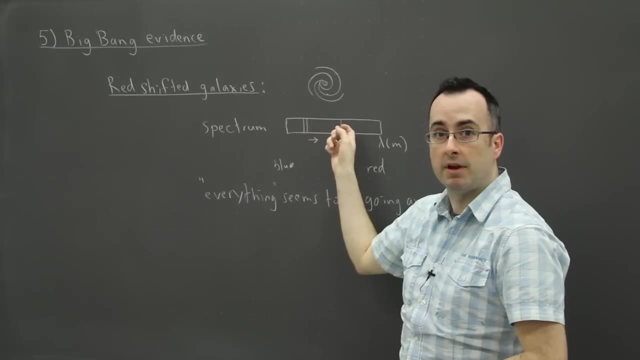 jumbling together in what we call a local group. But other than that, pretty much any other galaxy you look at, there's millions and millions of other galaxies. they're all going away from us. In other words, the light is all red shifted. 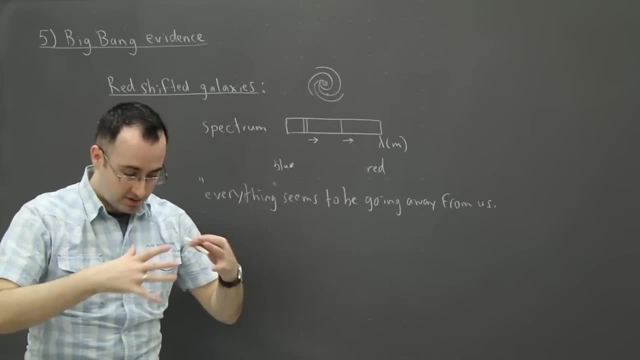 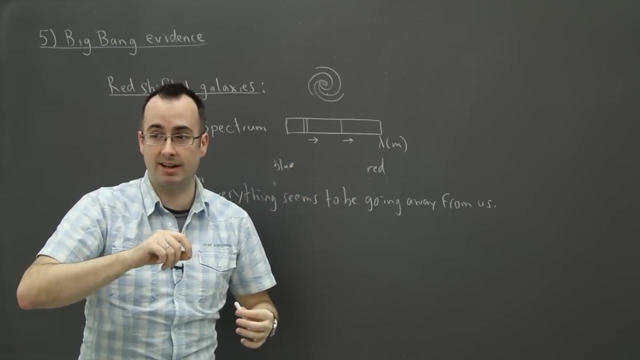 So the only explanation that we can come up with that makes sense: if everything is going away from us must mean that the universe is expanding. That or we're at the center of the universe and we really stink and everybody hates us because everything's going away. 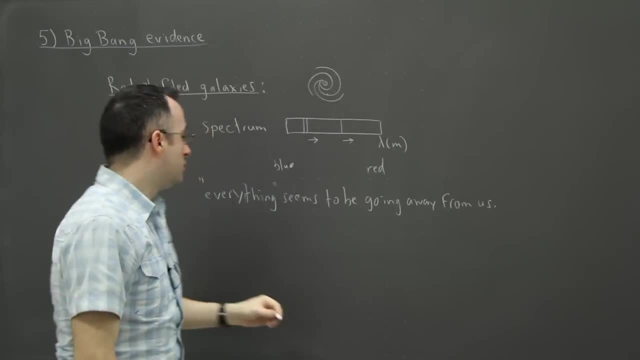 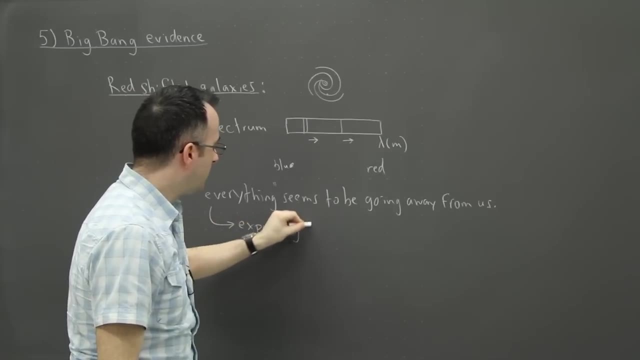 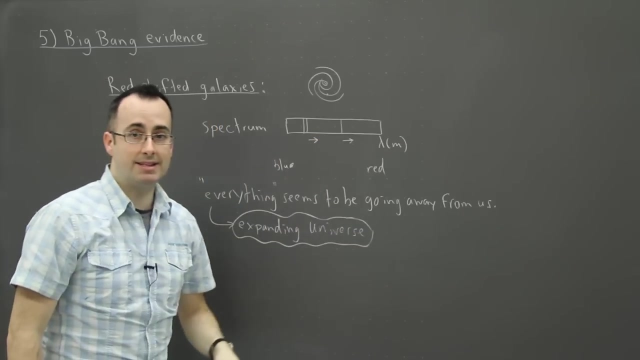 So the other explanation is that everything is expanding. So this tells us, then, that expanding universe. that's the conclusion that we can make from this. Okay, that's the. that's what red shifted galaxies tell us: that the universe must be expanding. 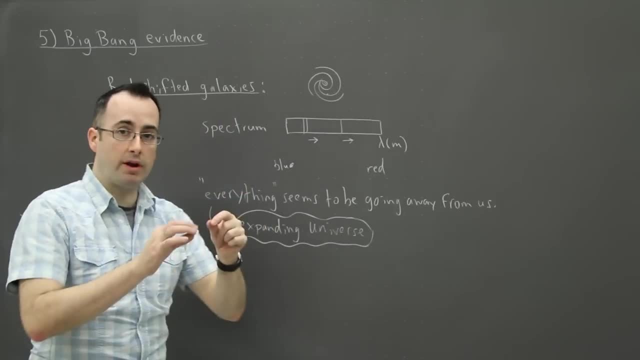 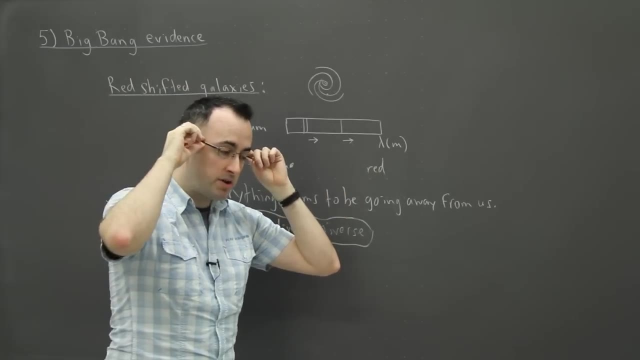 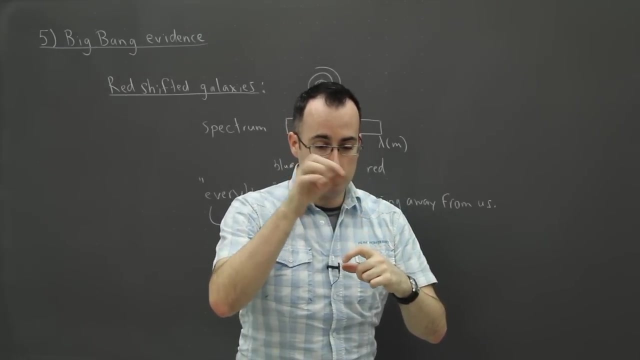 One way to understand how we think that every point or every galaxy from every other galaxy is increasing in distance, And a simple way to try to understand that is. imagine you take a balloon and you're going to blow it up with air. Well, what you can do is on that balloon. 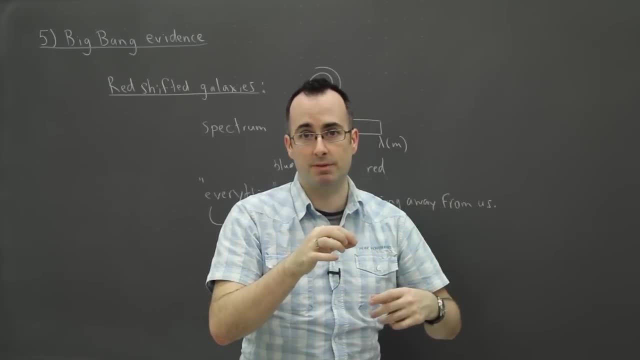 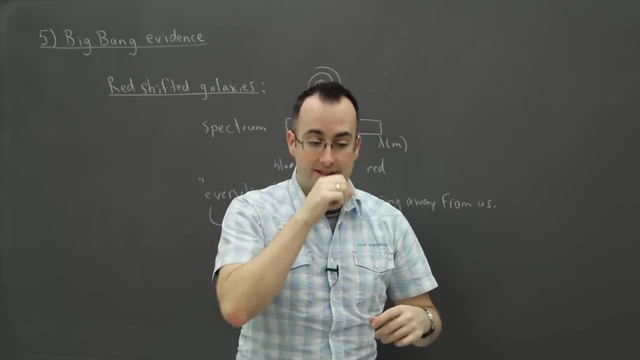 I mean, this is a bit of a. this is a tried and maybe tired explanation, but this one works. You take a balloon and you put a bunch of dots. like with a marker, you put dots on the balloon. What you do then is, as you blow it up, the distance from every dot to every other dot is going to increase. 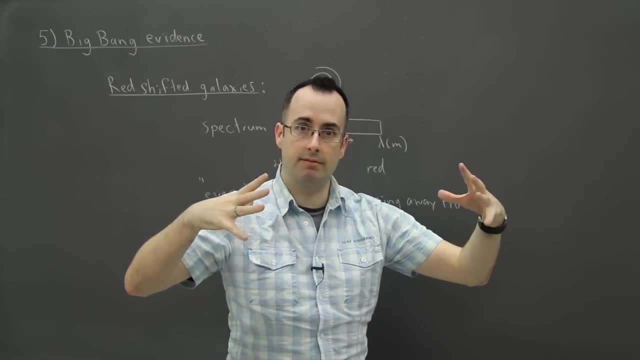 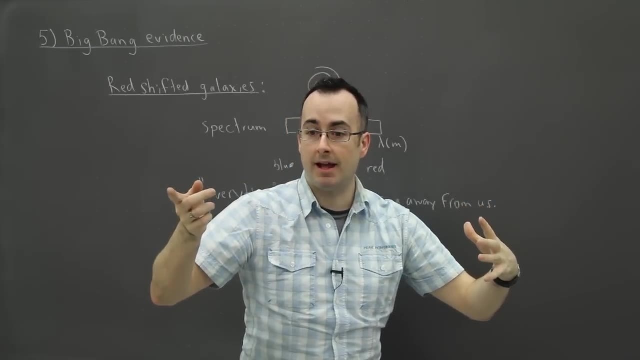 And that's what we think is happening- is that everything's increasing in distance because the universe is expanding. Now the question might be: expanding into what? And that's something we don't really have an explanation for. The universe isn't really expanding into anything. 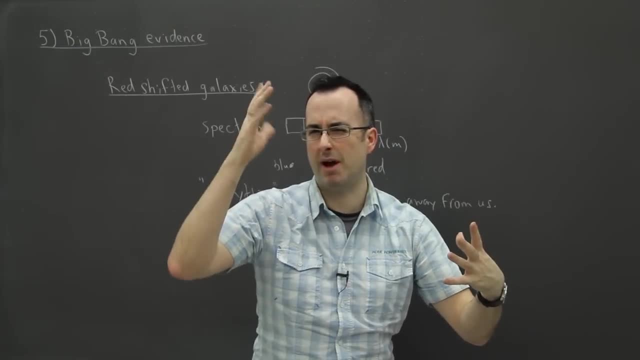 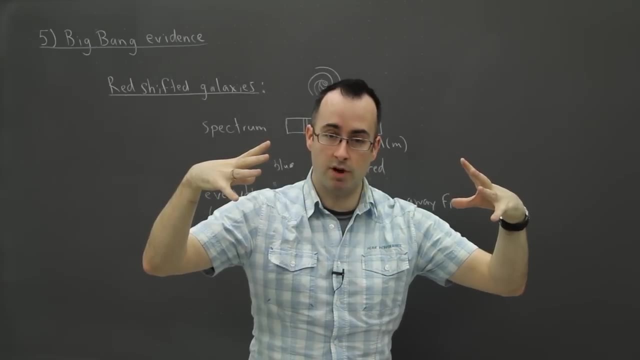 Everything we imagine is part of the universe. That's hard to wrap our brains around. Also, if the universe is expanding, it's pretty logical to think: well then what if we reverse time? Maybe at some time everything was in the same place. 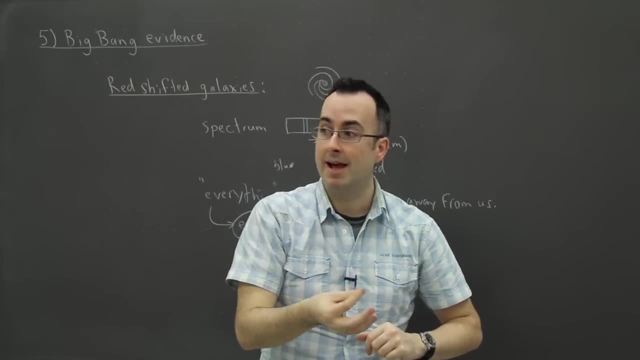 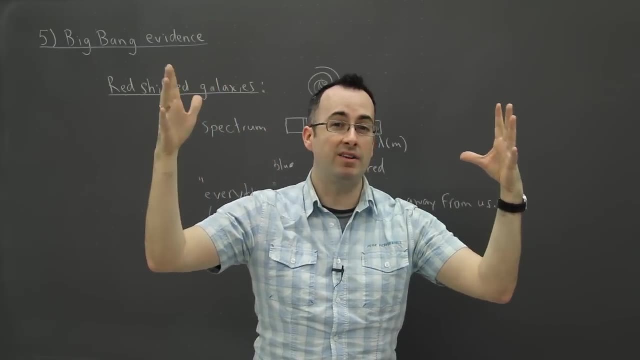 In other words, maybe the universe was all at one point. That's why it's called the Big Bang Theory, because something must have caused everything to expand. Now, what caused this? We don't know What happened before the Big Bang. Don't know What's at the other side of the universe. Stupid question. 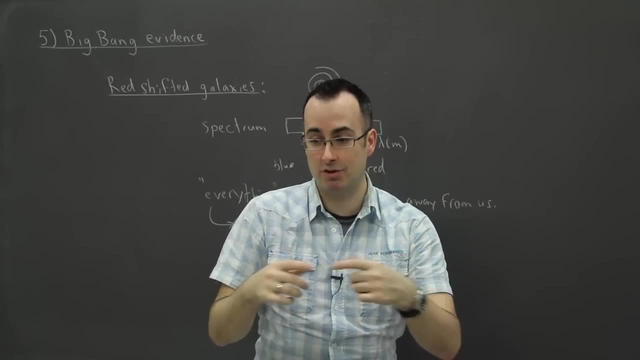 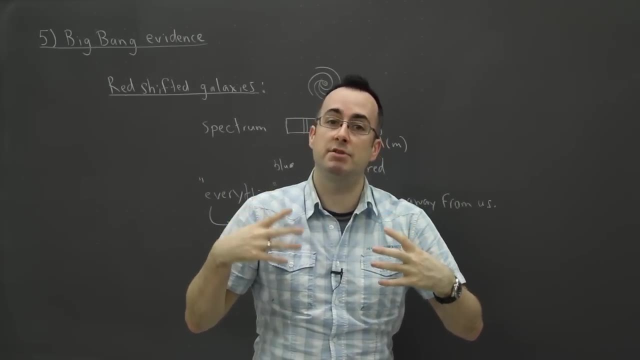 There is nothing on the other side of the universe by definition, because if you knew what it was, it's part of the universe, It's anything. So there's some problems, or at least some some conceptual issues with the Big Bang Theory. 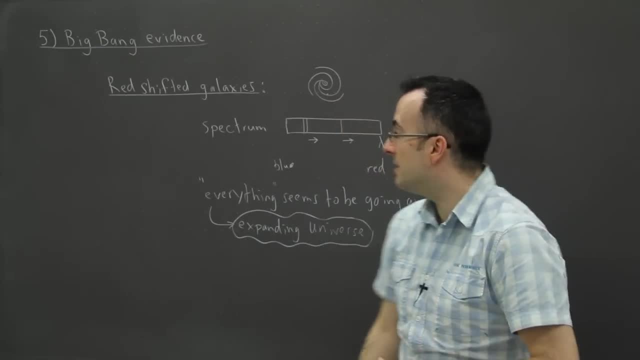 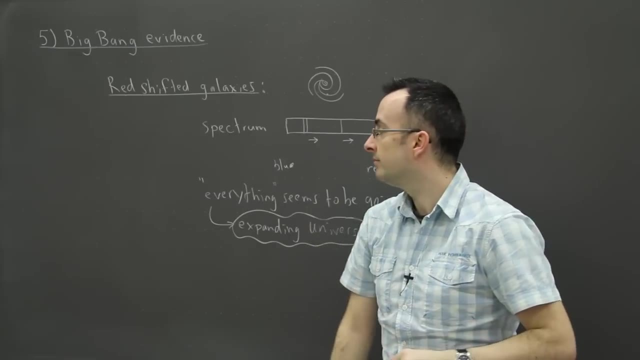 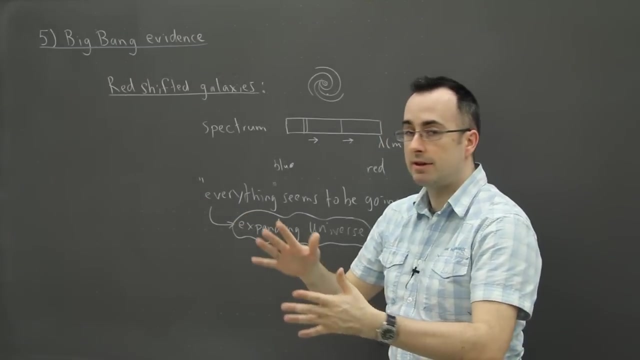 It's hard to wrap our puny little brains around this stuff, but the evidence seems to show that the universe is expanding, So it's natural to think that things started off as a Big Bang. In fact, cosmologists have really good theories for how exactly things happened from then on, so we've got lots and lots of evidence that seems to show that this is the case. 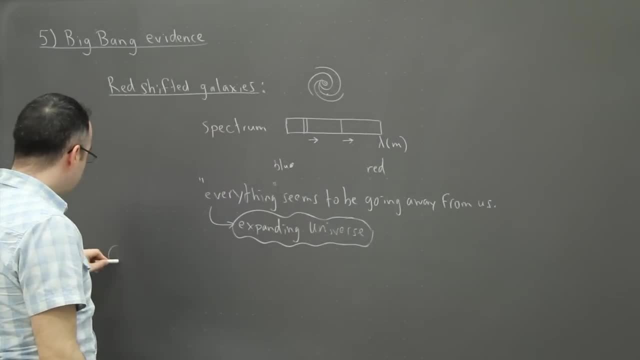 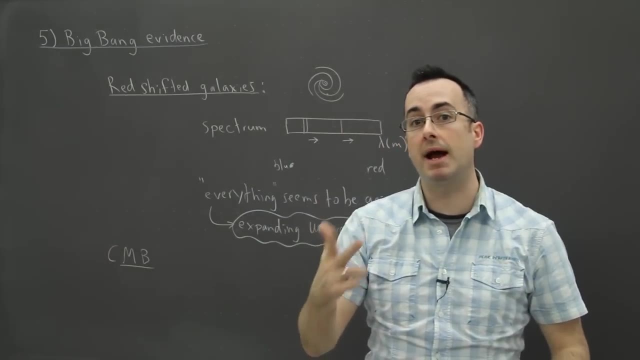 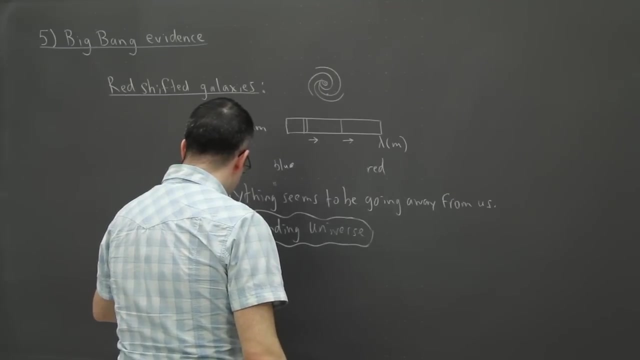 And another piece of evidence is cosmic microwave background. Okay, so that's what CMB stands for: Cosmic Microwave Background Radiation- And this- this is the key thing right here to learn- is this temperature right here: Temperature of 2.7 degrees Kelvin. 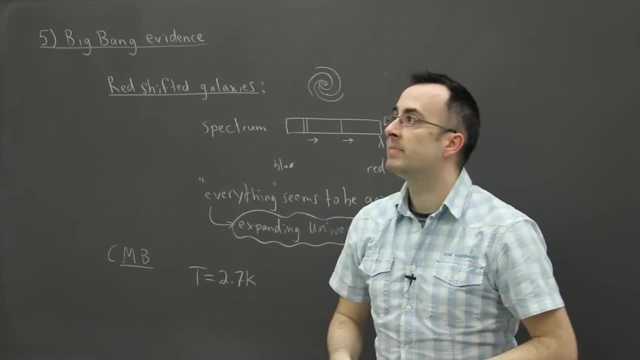 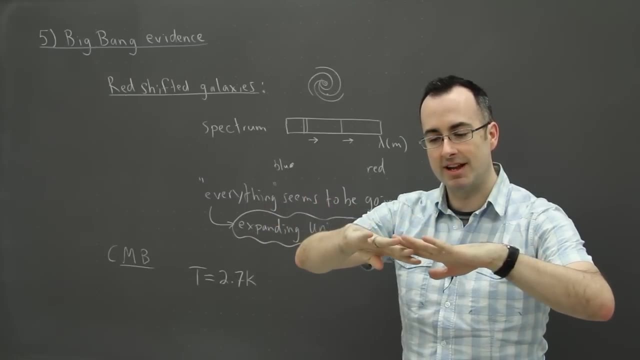 Now what this means, or what this represents, is it's like. it's like two different teams of people were looking at different things and didn't realize at first that they're actually sort of explaining each other. So people who were calculating: okay, what happened with the Big Bang? 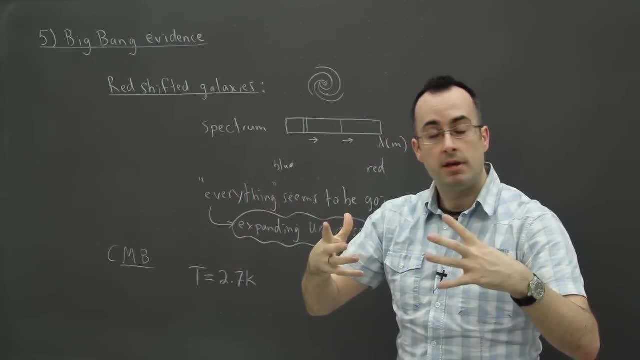 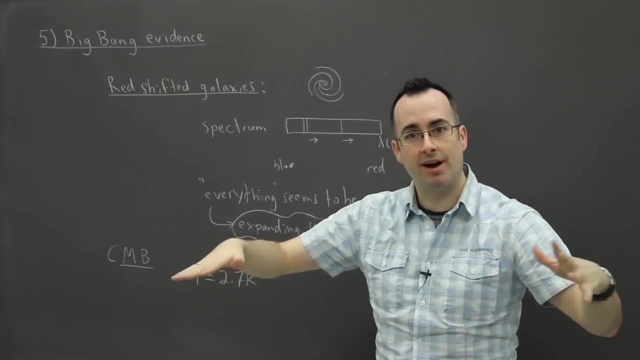 If there was a big explosion it should have been very, very bright, And from there then they could calculate: well, how bright should it look? now You know an explosion, you know sort of dims over time. So with some estimates they figured: ah, you know the temperature. 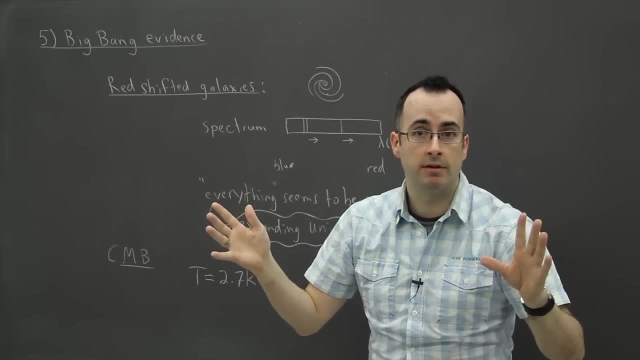 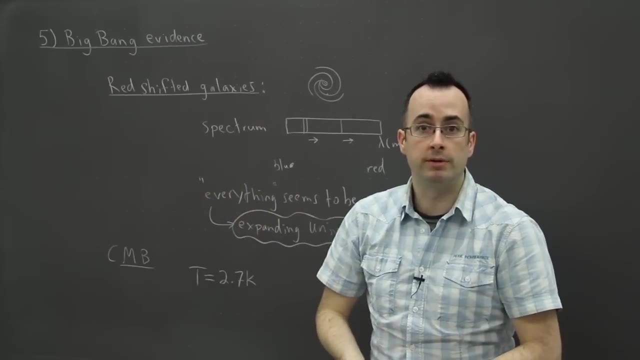 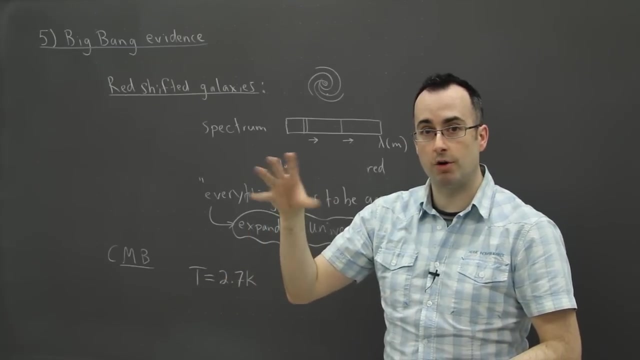 the temperature of the universe should be around three degrees Kelvin. This is what they figured a while ago. They just calculated this, said yeah, universe should be around three degrees Kelvin, but who knows? Then along came two guys named Penzias and Wilson and they were working with a radio telescope. 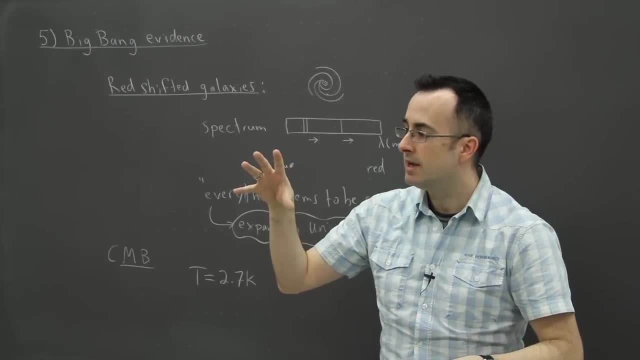 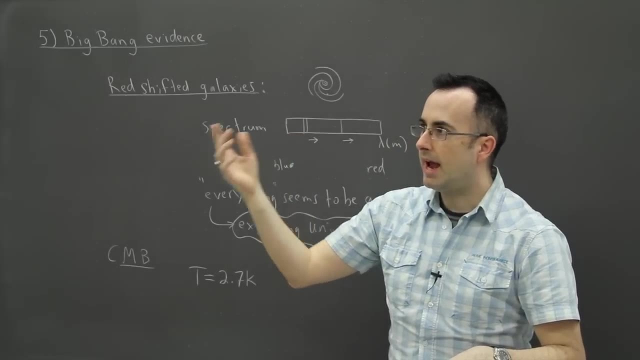 So this is a long time ago, when they were still just just starting with these, And when they're looking around, they noticed that they were doing something totally different, by the way, And with their radio telescope, everywhere they pointed, they always got an annoying signal. 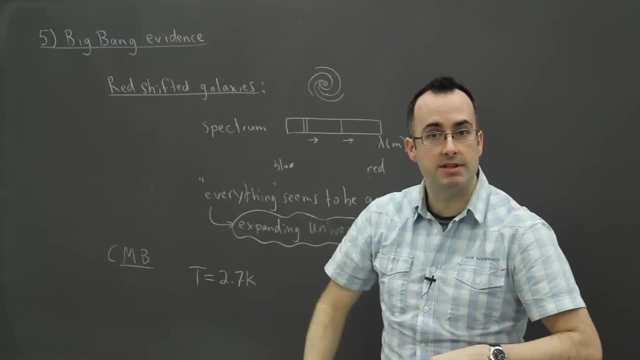 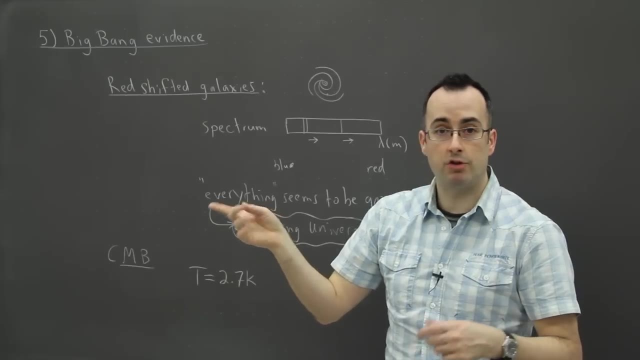 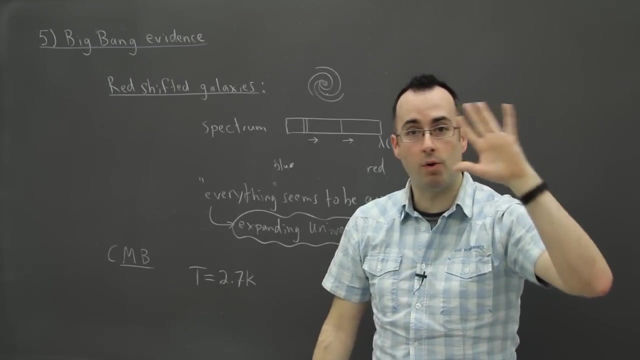 They thought that it was some sort of weird error or some weird bug in their system and it turned out that signal corresponded to what we call a temperature of around two point seven degrees Kelvin. So Penzias and Wilson had this annoying background radiation that they always detected everywhere they looked in the sky. 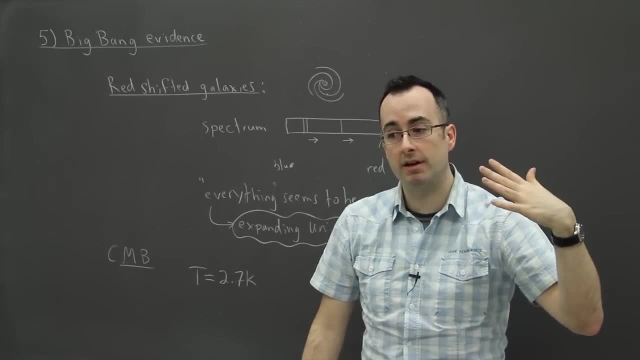 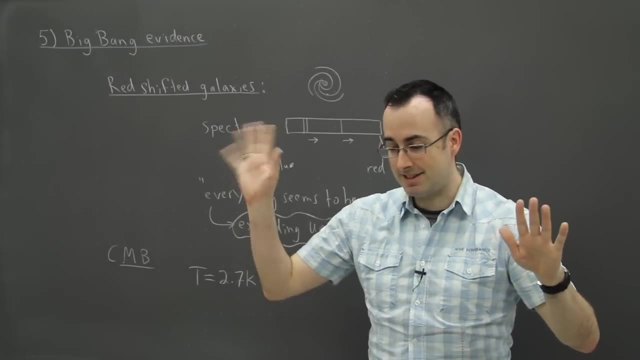 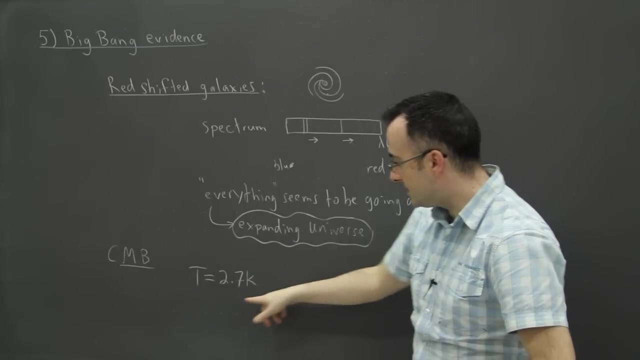 seemed to always have this same amount of radio wave emission, corresponding to around two point seven degrees Kelvin. And it turned out that that and this theory that the universe's cooling should be around 3 degrees Kelvin- look how well those two match up. So this piece of evidence here, the fact that everywhere you look, 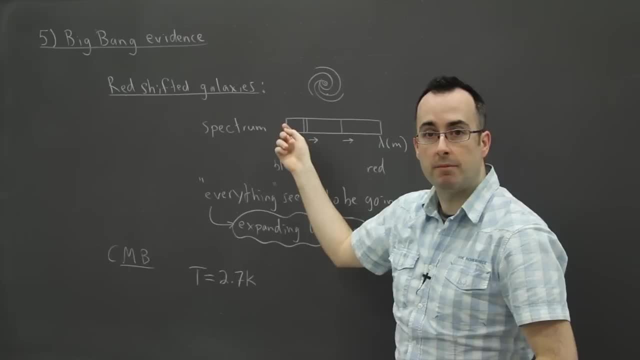 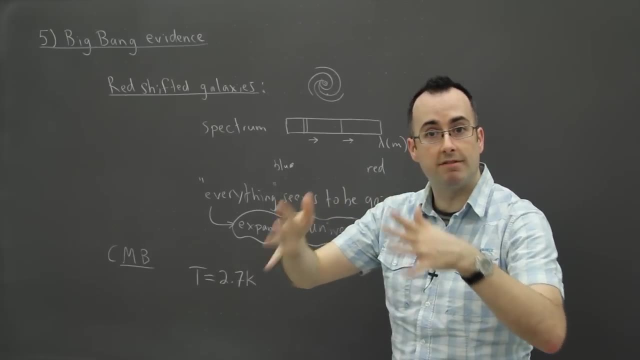 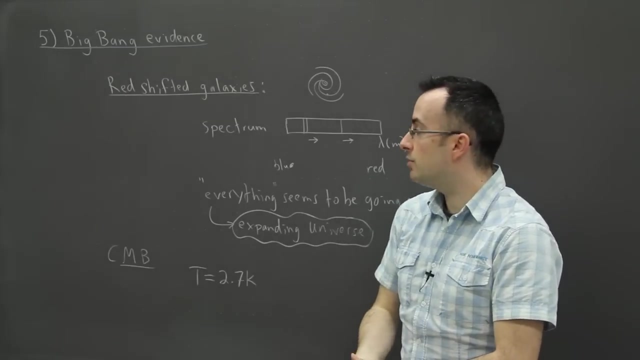 not only do you see galaxies going away from us, but you also see this temperature left over, this sort of left over from the cooling of the Big Bang, And everywhere you look you always see this 2.7 degrees Kelvin. So the Big Bang theory explains these really well, plus a whole bunch of other things. 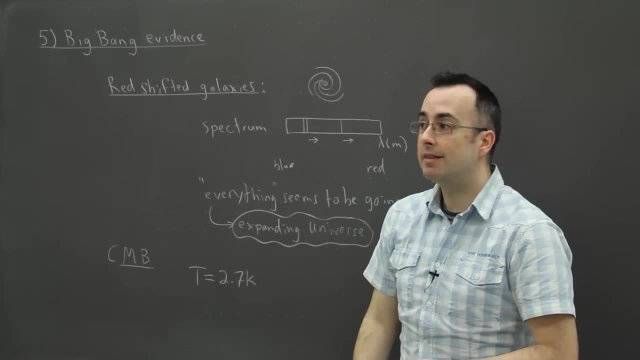 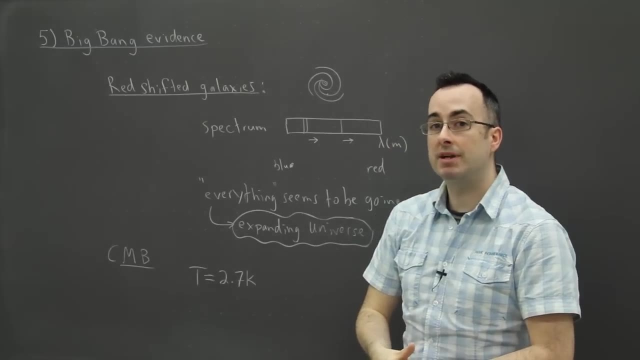 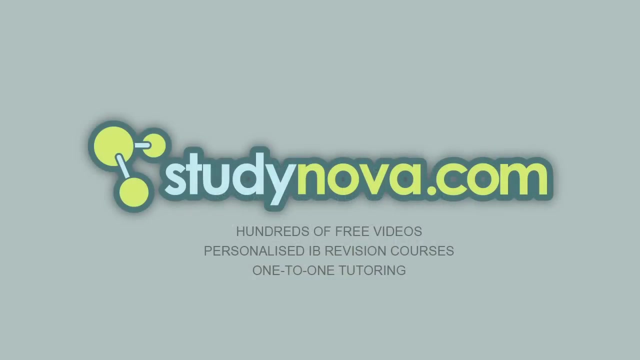 And that's why, even if you don't like it, I think you need to accept it, because evidence really seems to point towards it. So any other theory of the universe had better explain these two facts, because these are observational evidence. Subtitles by the Amaraorg community.